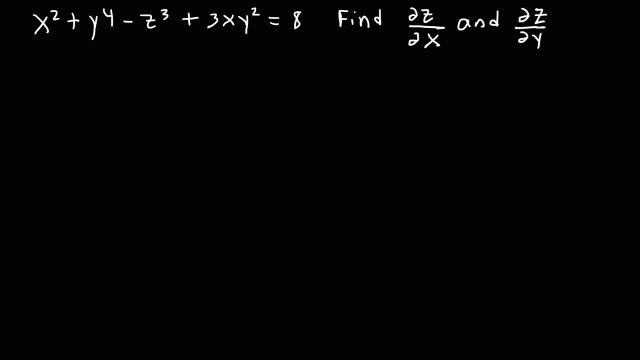 So here we have an equation in terms of x, y and z, And we're asked to find the partial derivative of z with respect to x and the partial derivative of z with respect to y. Now we're going to use the implicit function theorem to get the answer, And then we're going 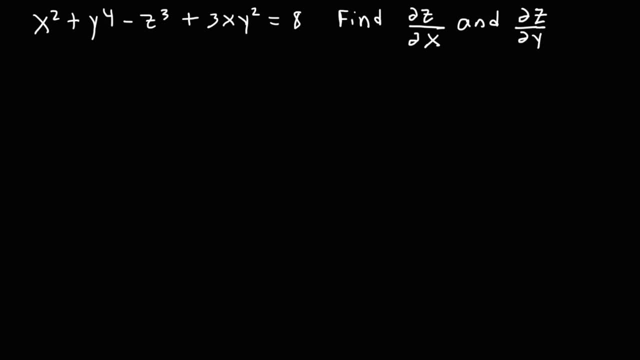 to talk about another way that we can get the answer. So let's go ahead and begin. The first thing we want to do is move the 8 to the other side So we can get a 0 on the right side, And we're going to represent that as f of x of y. I mean f of x comma y. So that's going to be. 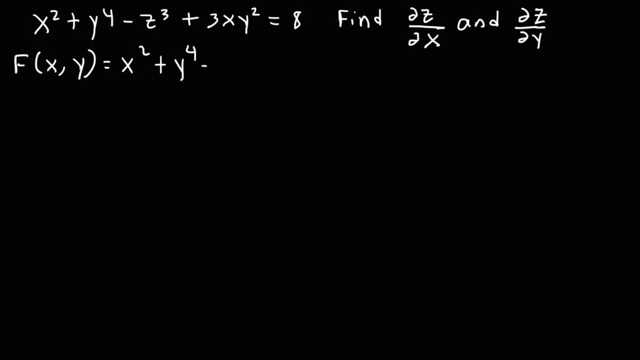 x squared plus y to the fourth, minus z to the third, plus 3xy squared minus 8, which is equal to 0.. So once you have this function, you want to find the partial derivative with respect to x. So the derivative of x squared will be 2x. We're going to treat y as if it's a constant And the 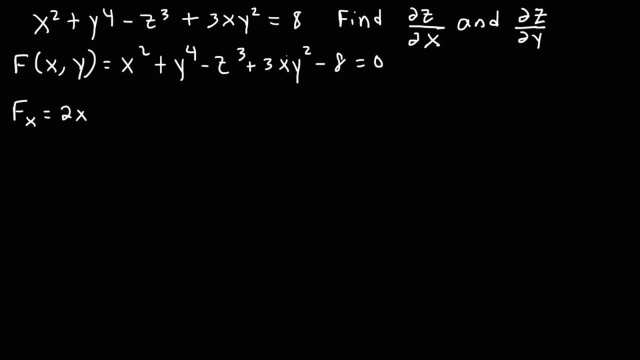 same is true for z, So that's going to become 0.. Now this has an x in it, So the derivative of x is 1. And the derivative of the constant negative 8, that's 0.. So f of x is 2x minus 3y squared. 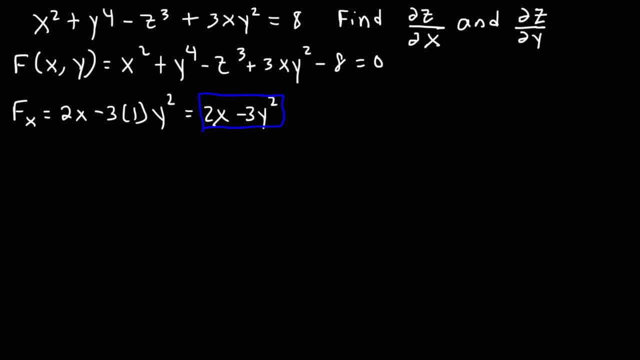 So we're going to save that for later. Let's find the partial derivative with respect to y. So the derivative of y to the fourth is 4y cubed, The derivative of these two. we're going to treat them as constants, So they're going to be: 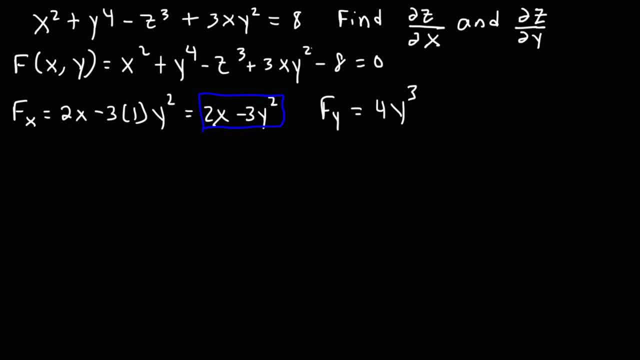 0.. Now for this one. we're going to treat the 3x part as a constant, But we're going to take the derivative of y squared, which is 2y, And so this is going to give us 4y cubed plus 6xy. 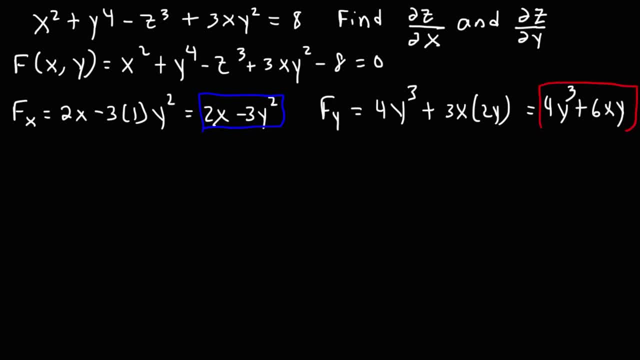 Now I noticed that I made a small mistake. This should be positive and not negative. So now let's move on to f sub z. The only term with a z variable is this: The derivative of x squared y to the fourth, 3xy to the second power and negative 8, all of that is going to be 0.. 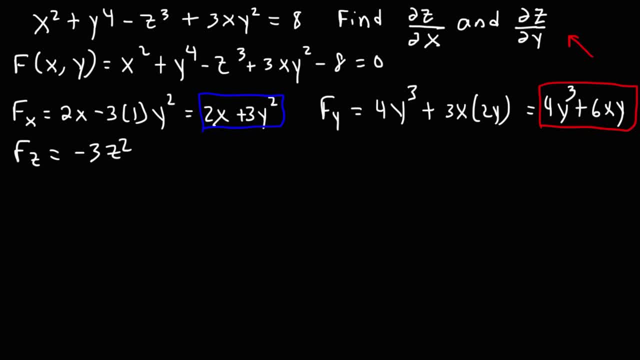 So f sub z is going to be negative, 3y cubed z squared. So now that we have that, we can calculate the partial derivative of z with respect to x. So this is going to be z sub x. z sub x is equal to negative f sub x over f sub z. So that's negative times 2x plus 3y squared. 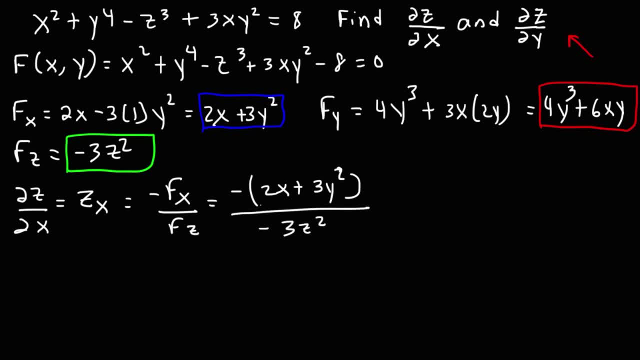 divided by negative, 3y, 3z squared. So we can cancel out the negative sign, giving us this answer: 2x plus 3y squared over 3z squared. So that's the first answer. That's the partial derivative of z with respect to x. 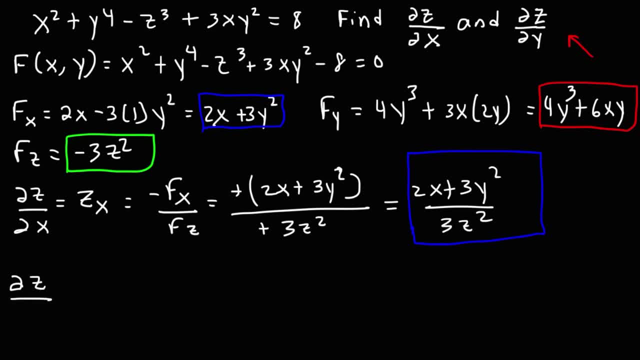 Now let's calculate the partial derivative of z with respect to y. So that's going to be z sub y and that's equal to negative f sub y over f sub z. So f sub y is 4y cubed plus 6xy and f sub z is negative 3z squared. Once again, we can cancel. 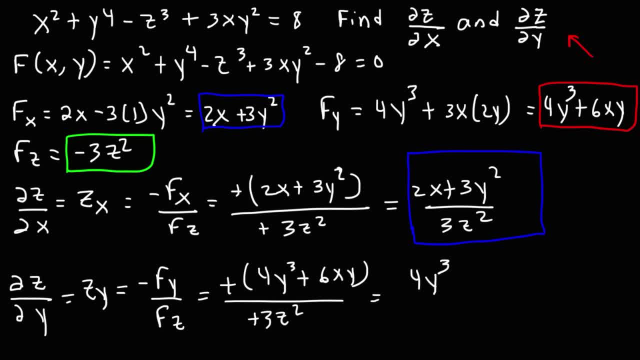 the negative sign, And so it's going to be 4y cubed plus 6xy over 3z squared. So that's how we could use the implicit function theorem to get these two partial derivatives. Now let's use another method to get the same two answers. 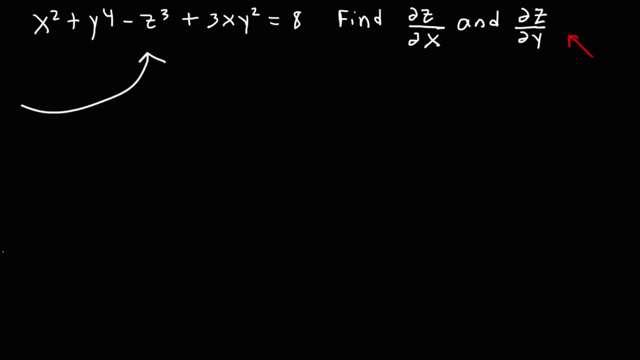 So we're going to use implicit differentiation on this equation, So let's find this one first. So we need to find a partial derivative of z, or, for some reason, we need to find a partial derivative of z. So we need to find a partial derivative of z, or, for some reason, we need to find a partial derivative of z. 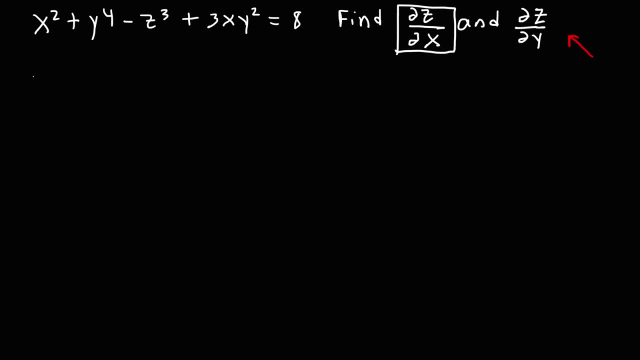 When we differentiate x squared with respect to x, it's just going to be 2x. Notice that there's no y variable in that expression. So we're going to treat y as if it's a constant. The derivative of y to the fourth is going to be 0.. Now when we're 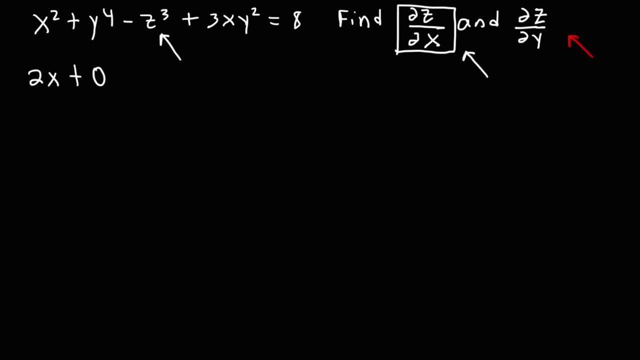 differentiating a z variable, we're going to add the partial derivative of z with respect to x. next to it, The derivative of negative z to the third power is negative 3, z squared, and then it's going to be times the partial derivative of z with respect to x. 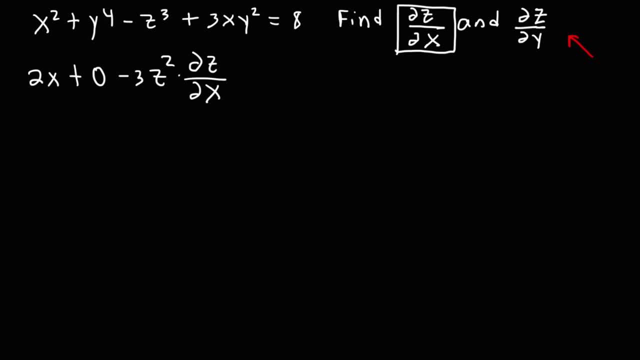 Now for this one. the 3 and the y squared are constants, So all we need to do is differentiate x, So it's going to be 3 times 1 times y squared, And then the derivative of 8 is going to be 0.. 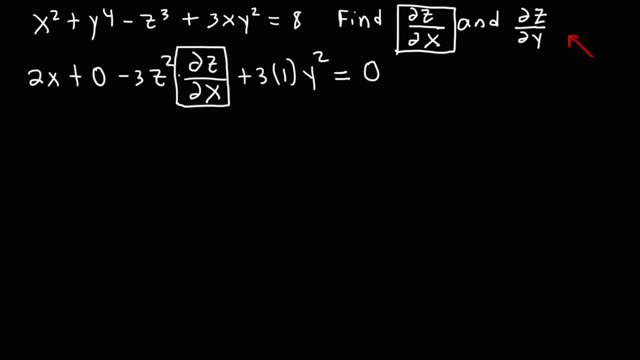 So now what we need to do is isolate this variable So the 3 and the y squared are constants. So we're gonna have negative 3, z squared times the partial derivative of z with respect to x, And that's going to equal negative 2x minus 3y squared. Now the next thing that we need to do 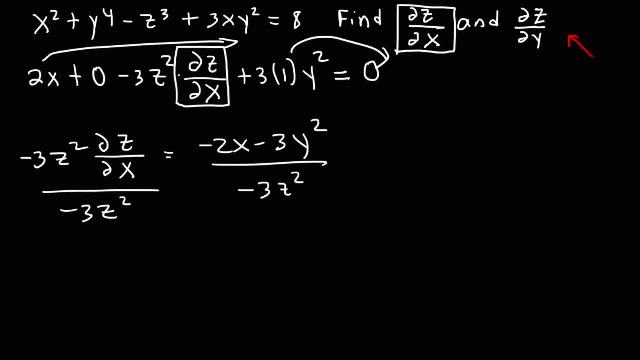 is: divide both sides by negative 3, z squared, And then we're going to factor out a negative sign in the numerator. So it's going to be negative 2x minus 3y squared, And then we're going to factor out a negative sign in the numerator. 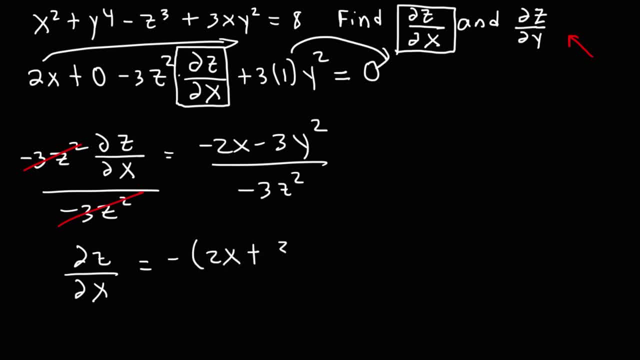 So it's going to be negative. and then 2x plus 3y squared over negative 3z squared, and now we could cancel the negative sign. so thus this is going to give us the answer that we had before: 2x plus 3y squared. 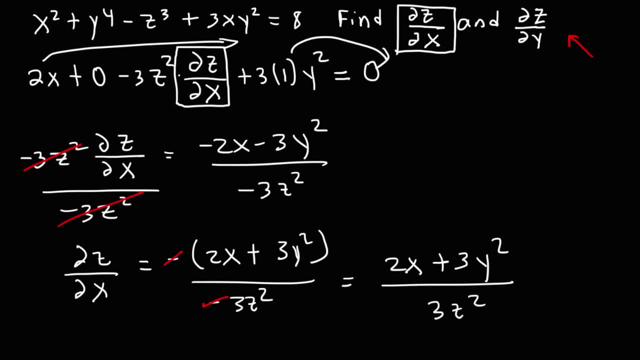 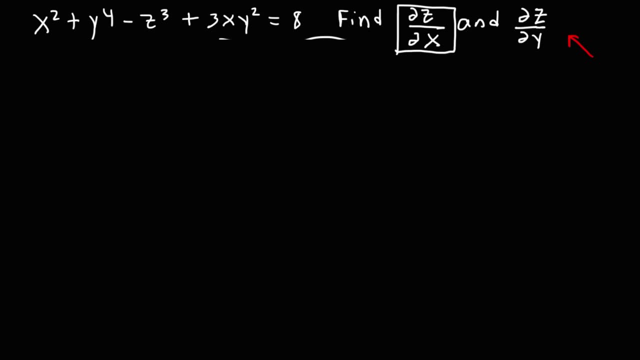 divided by 3z squared. so that's another way in which you can get the same answer. now let's find the other answer, the partial derivative of z with respect to y, using the same process. so we're going to treat x as if it's a constant. so once we take the derivative of that, 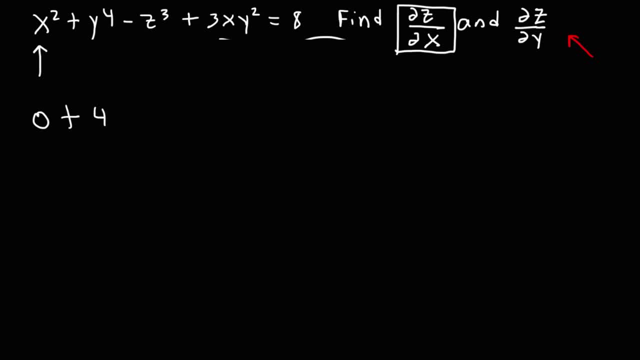 that's going to be 0. the derivative of y to the fourth will be 4y cubed and the derivative of z to the third will be 3z squared but times the partial derivative of y to the fourth of z with respect to y. now the 3x will be treated as a constant, but we're going to differentiate. 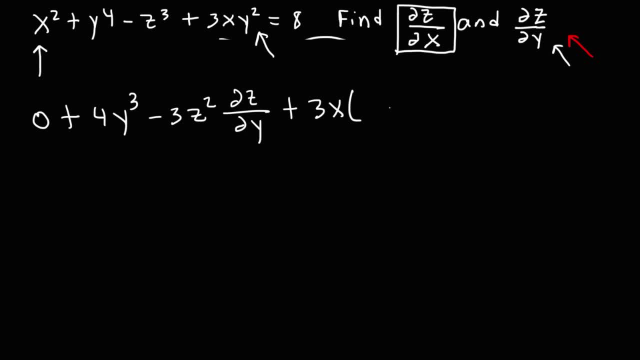 the y squared part, since we have y in that expression. so it's going to be times 2y equal to 0. so let's move this term to the other side and the 4y cubed to the other side, so it's going to be negative. 3z squared times the partial derivative of z with respect to y, and that's. 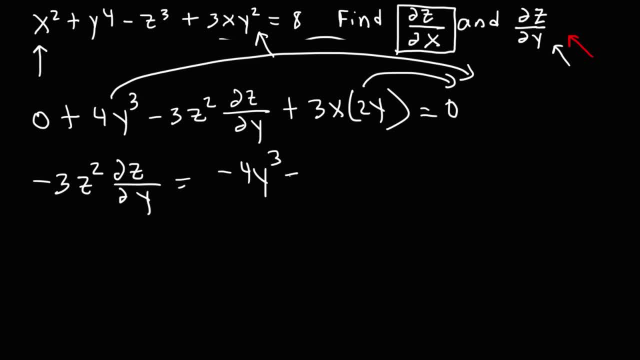 going to equal 3z, squared negative, 4y cubed minus 6xy, and then divide both sides by this, and so we have the partial derivative of z over the partial, i mean with respect to y, it's going to be negative. let's factor our negative sign again, 4y cubed plus 6xy, over this. 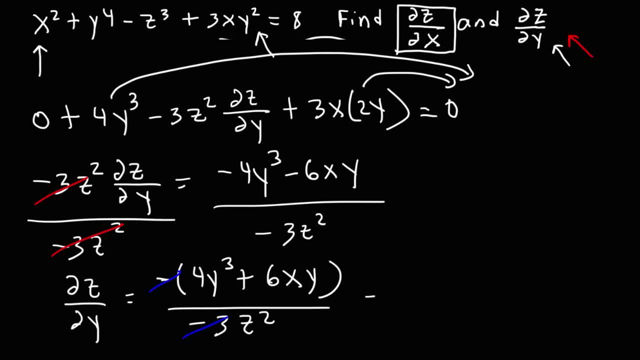 and then we can get rid of the negative sign. given us our answer: 4y to the third plus 6xy, all divided by positive 3z squared. so now you have two ways in which you can get these two partial derivatives. now let's work on another. 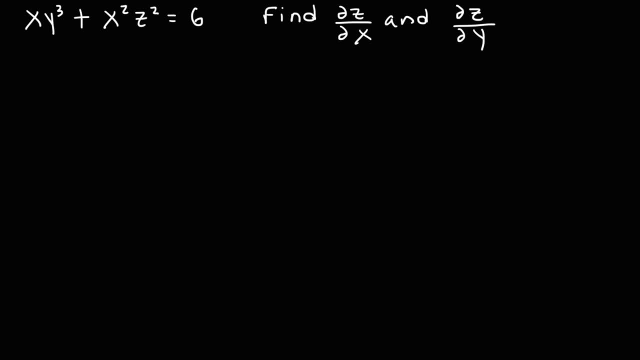 example, for the sake of practice, feel free to pause the video if you want to try it. so let's begin. let's begin by moving the 6 to the other side. so first to move this miracle BILLI energies up and the initial derivative of x to the other side of our graph, and then we're taking 2x to the other side. 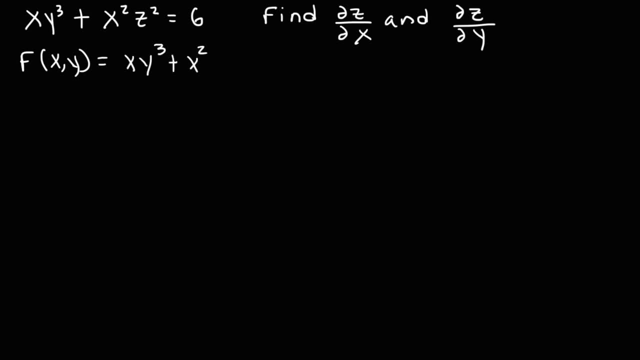 and we're moving about by dividing 5y and 5y minus 6y to the other side, so we can say that f x comma y is xy cube plus x squared z squared minus 6, which is equal to 0. so now let's find a partial. 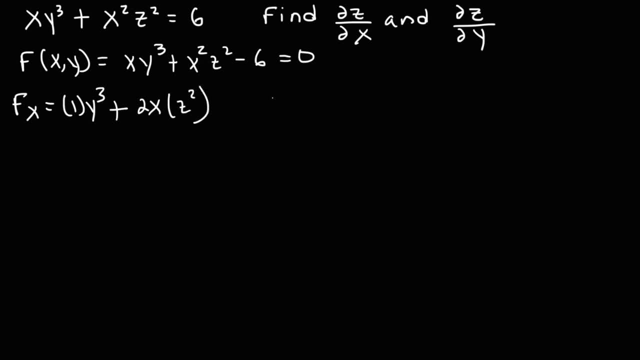 derivative with respect to x will be one. so this is going to be 1 times y cube and the derivative of x squared will treating y cubed and z squared as constants, and this will be 0.. So this is going to turn out to be y cubed plus 2x z squared. So now let's move on to the partial derivative with: 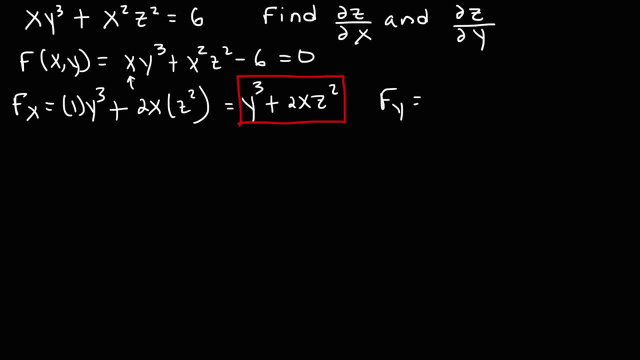 respect to y. So we're going to treat x and z as constants. The derivative of y cubed is 3y squared. This doesn't have a y variable in it, so that's going to be 0.. So it's just.